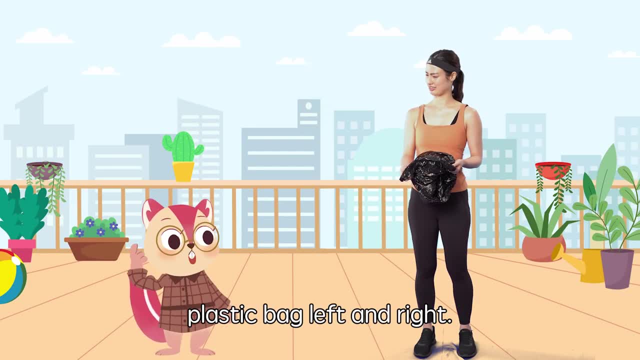 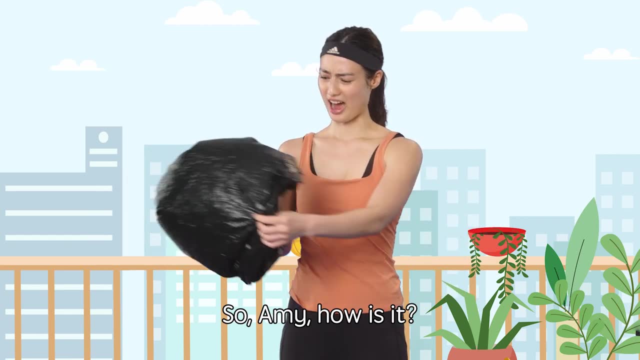 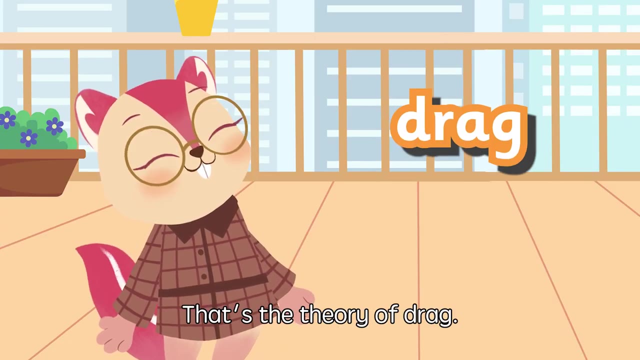 I want you to move this plastic bag left and right. Try it out. So, Amy, how is it? I can feel some kind of force dragging this bag. That's the theory of drag. Drag is the force that acts opposite to a relative motion of an object to make it slow down. 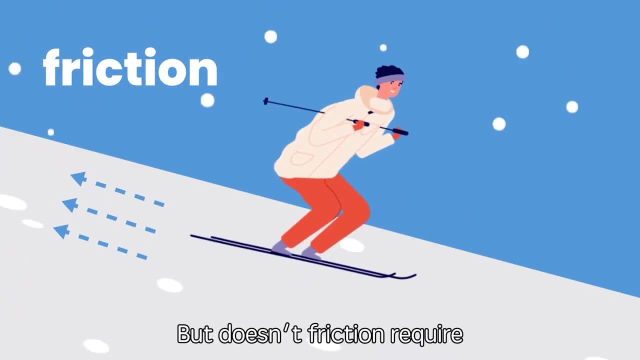 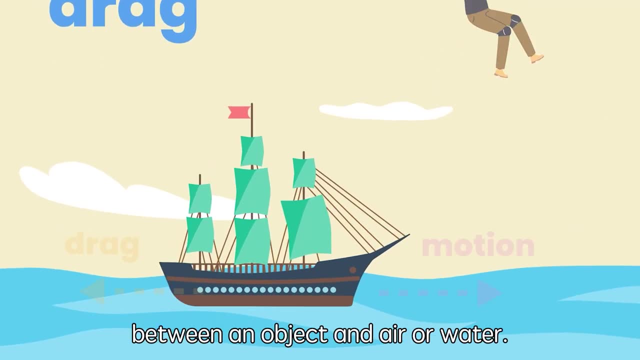 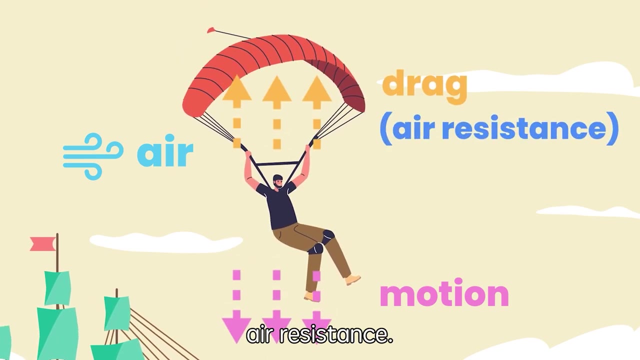 Hmm, this sounds like friction, But doesn't friction require two surfaces to touch? Drag is a type of friction between an object and air or water. For air, we usually call this air resistance. When you run, you can feel the air hitting on your face. 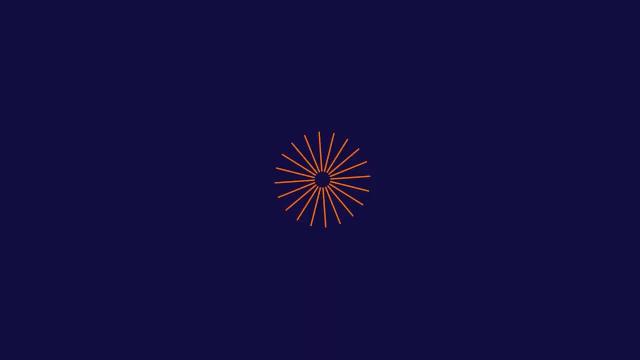 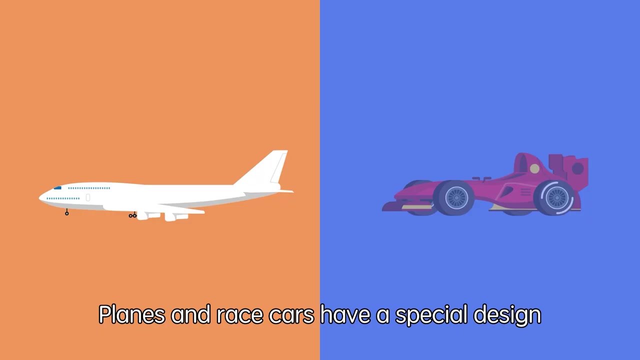 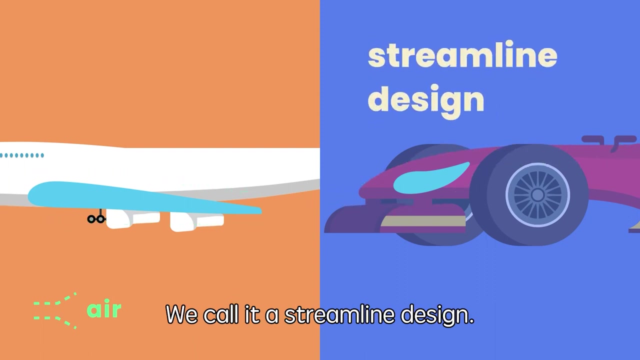 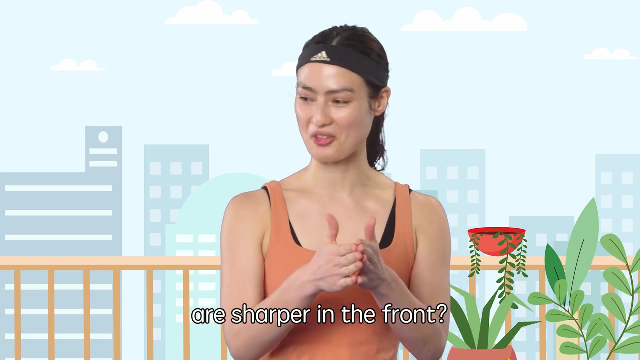 That is air resistance in action. Here's a fun fact: Chipsters, Planes and race cars have a special design. It's designed to reduce air resistance so it can travel at a faster speed. We call it a streamline design. Oh, is that why fast vehicles are sharper in the front? 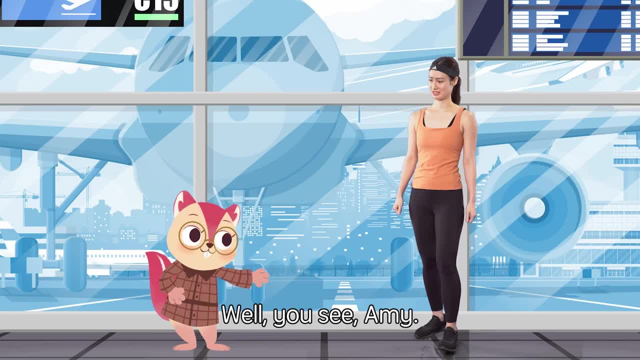 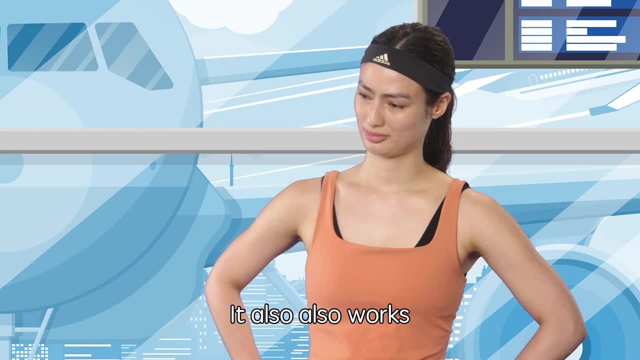 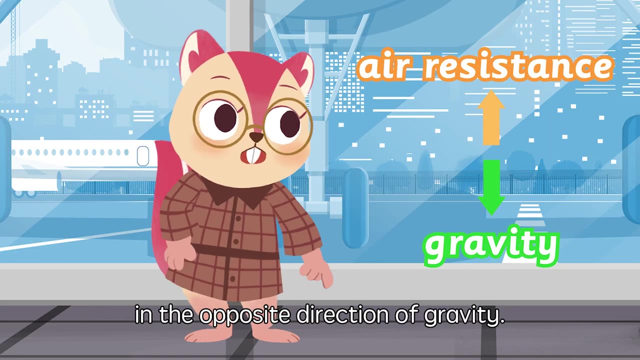 Ten out of ten. Amy, You're a natural. Well, you see, Amy, air resistance doesn't only work when we're moving horizontally, It also works when we're moving vertically, Meaning that it can act in the opposite direction of gravity. 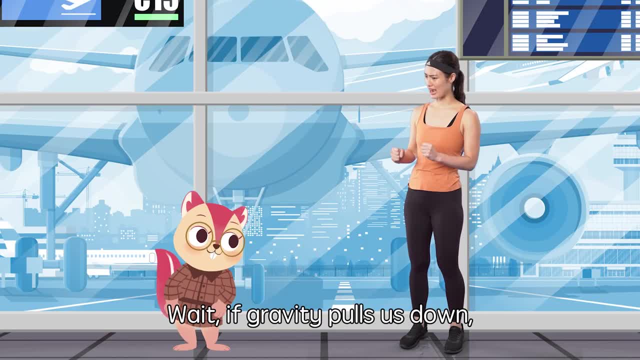 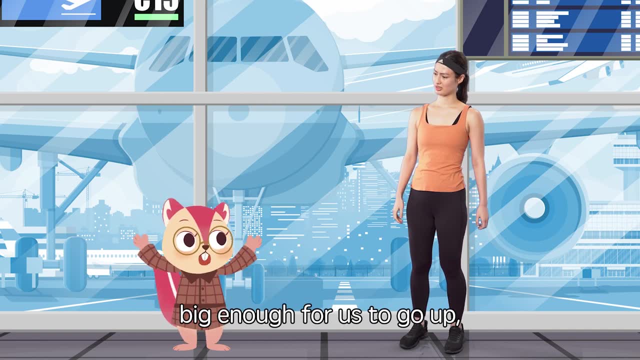 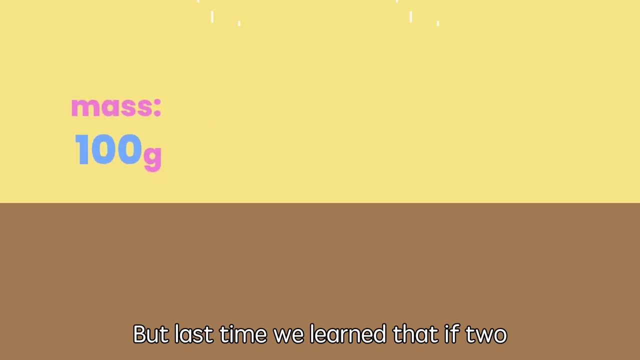 Wait, if gravity pulls us down, does air resistance pull us up? Well, Amy, air resistance would never be big enough for us to go up, but it can slow us down. Hmm, but last time we learned that if two objects have different mass, they will still touch the ground at the same time. 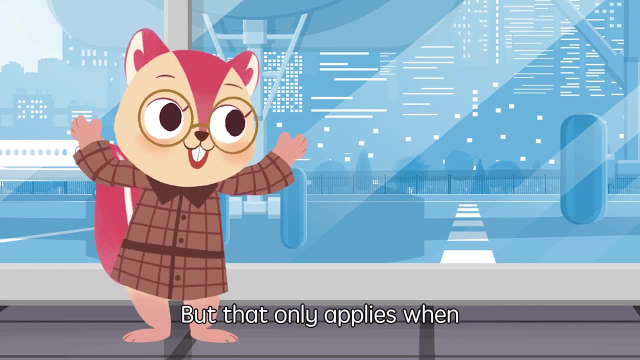 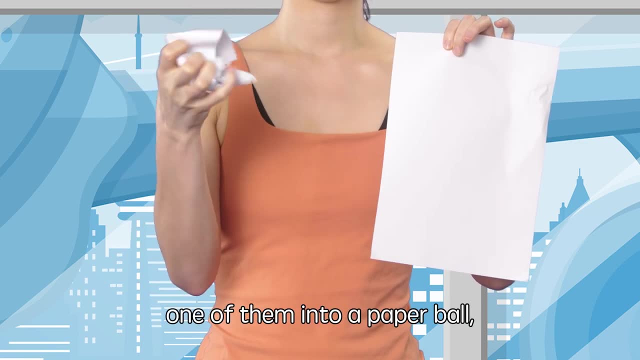 You're right, Amy, But what if two objects have different mass? But that only applies when there is no air resistance. Take these two same pieces of paper and crumple one of them into a paper ball, Then drop them from the same height at the same time. 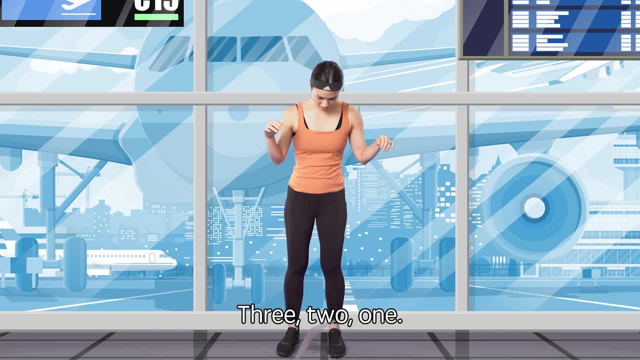 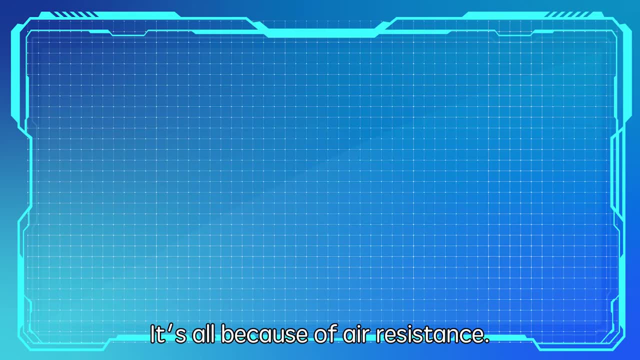 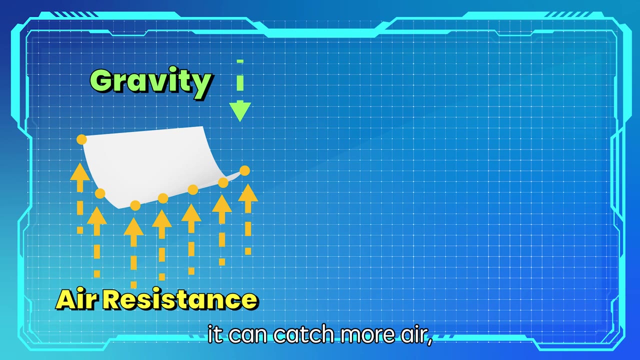 Three, two, one. The paper ball landed on the ground first. It's all because of air resistance. When we drop a piece of paper, it can catch more air, causing it to fall slower. The paper ball can't really catch air, so it fell faster than the piece of paper. 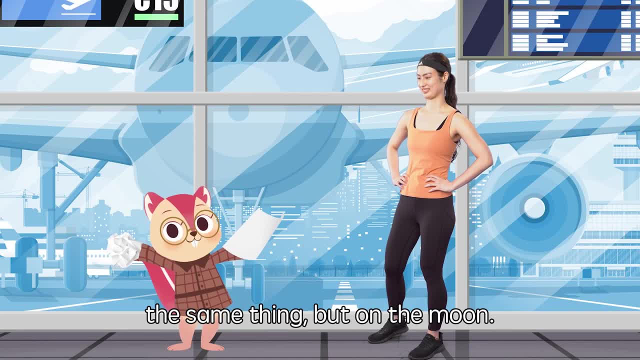 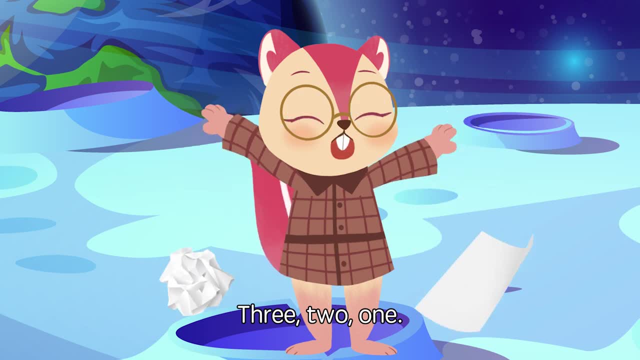 Now let's imagine that we do the same thing, but on the moon. Which one will hit the ground first? Chipsters Three, two, one. Wow, they both landed at the same time, But why? Oh, because of the air resistance. 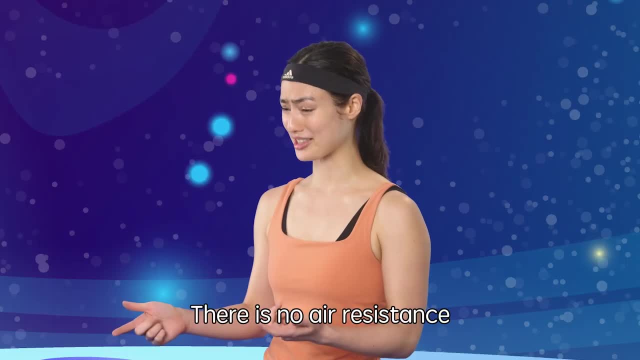 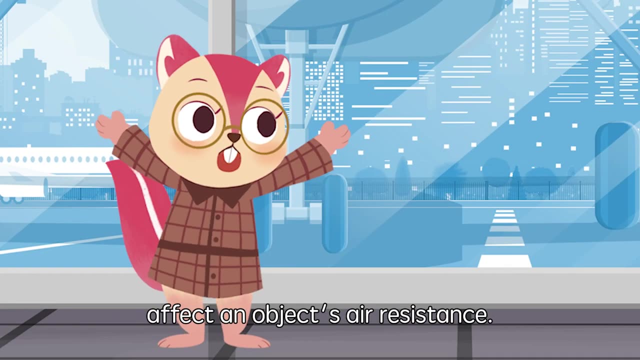 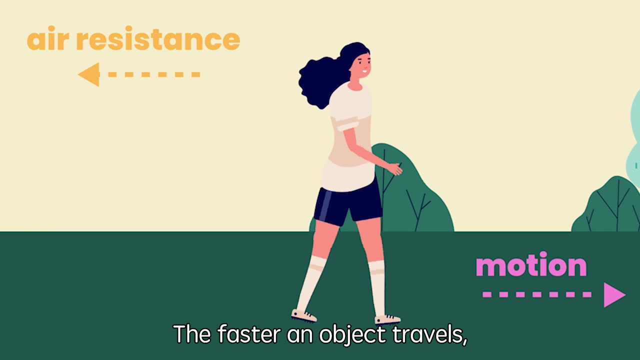 Because there is no air on the moon, there is no air resistance to slow the piece of paper down, Spot on. There are two factors that can affect an object's air resistance: The traveling speed of the object and its surface area. The faster an object travels, the more air resistance it experiences. 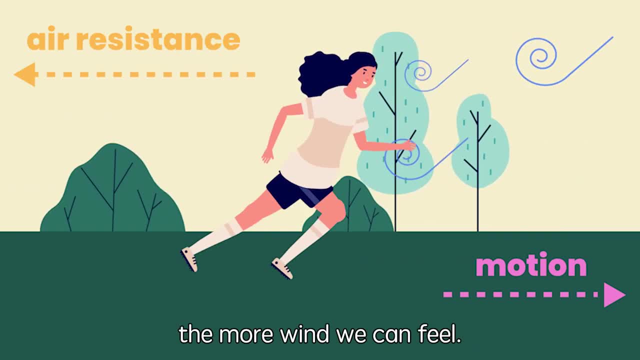 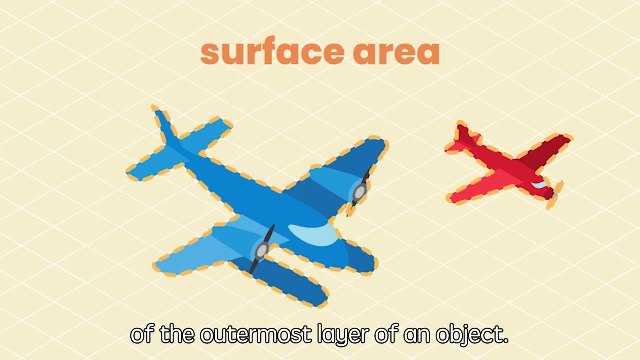 That's why the faster we run, the more wind we can feel. The surface area of the object is the area of the outer surface, The outer most layer of an object. the larger the object, the more air resistance it experiences. For example, this blue plane has a larger surface area than that red plane. 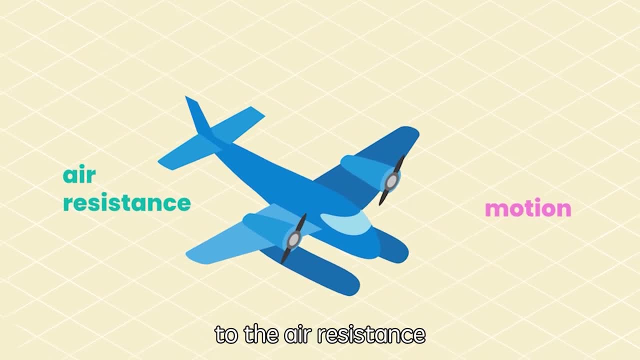 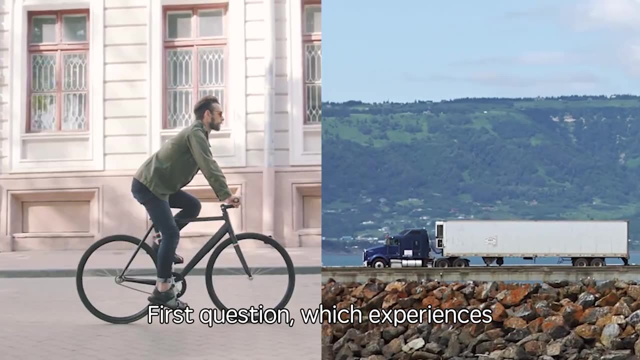 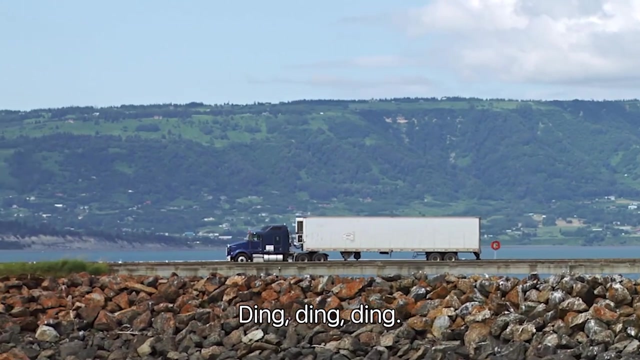 When the force of motion is equal to the air resistance, the object will move at a constant speed, meaning it won't go any faster. First question: which experiences more air resistance? a bicycle or a truck? Ding, ding, ding, Because a truck is bigger and has a larger surface area than a bicycle. 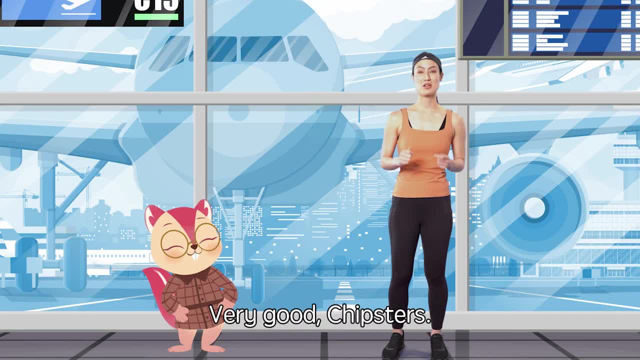 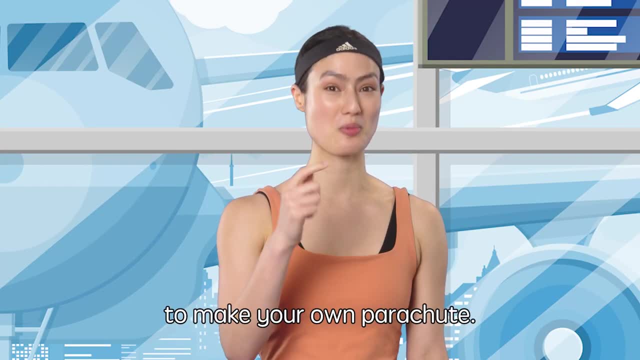 the truck would experience more air resistance. Very good, Chipsters, It's your turn to try it now. Join my experiment to see how to make your own parachute. Want to watch the full video? Sign up now and get started with your own free trial.